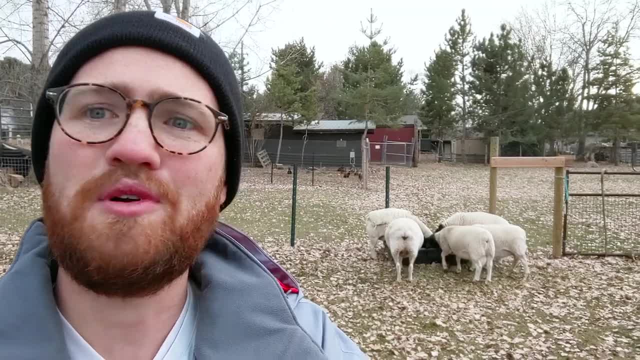 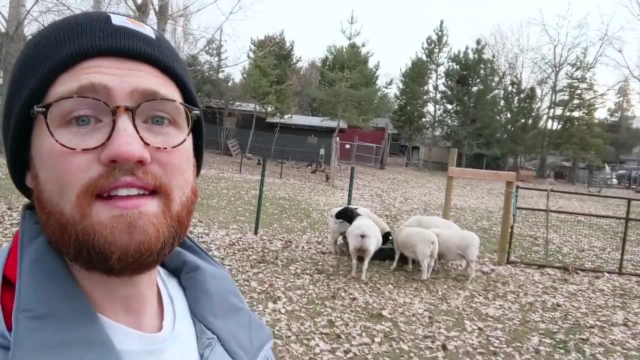 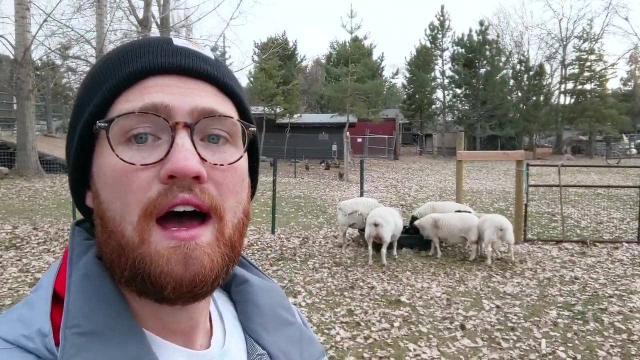 I don't really know where that stereotype comes from, which is why this video is here to talk about, uh, the truth behind it. Okay, So let's get down to it. Is sheep meat? is it called lamb or mutton? The answer is yes, It's both. Uh, so the general 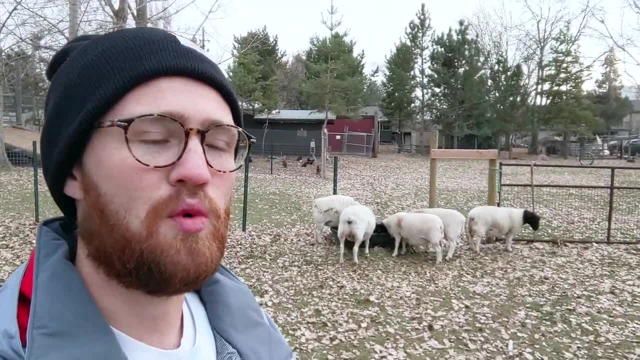 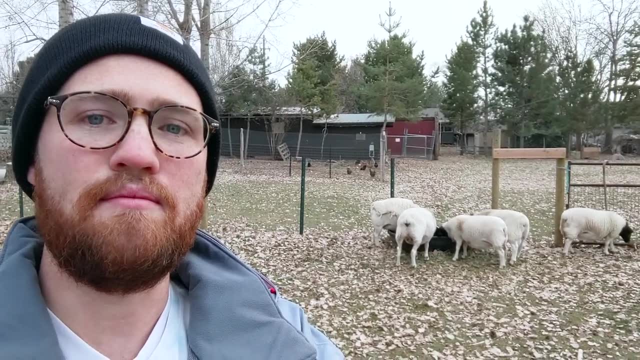 rule of thumb is that true lamb meat is anything processed where it is under a year of its life, And so I have a lot of friends that are interested in my lifestyle but not necessarily interested in the in the animal processing part, which I don't blame them for, And some of them 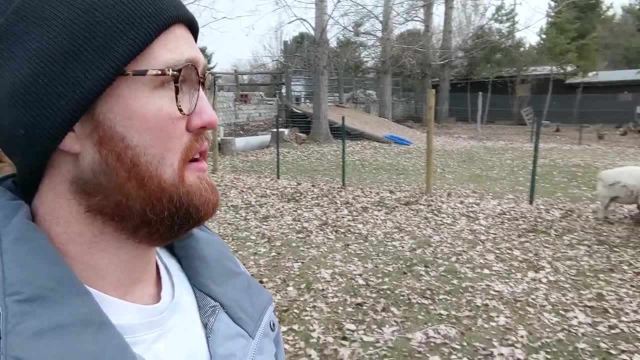 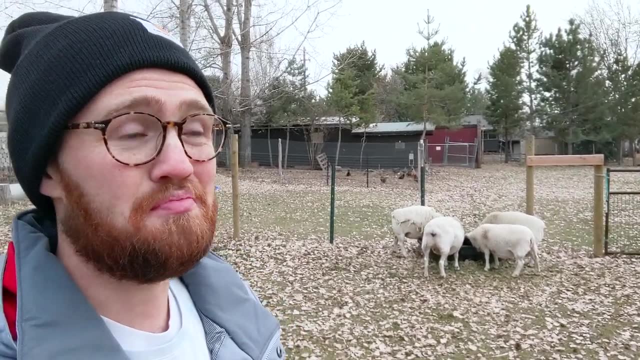 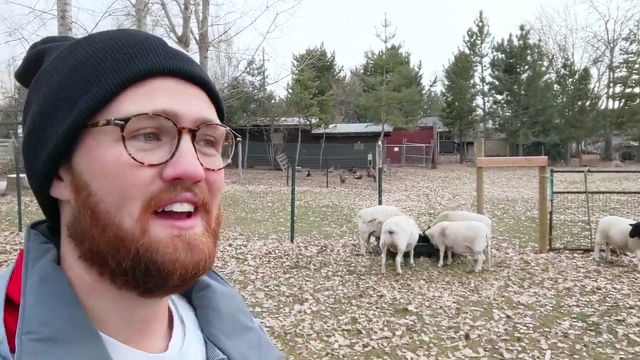 kind of think. maybe it's, it's cruel when you think about you know. Oh, you know they're lambs, they're babies, but I hate to break it to you. Every animal that you buy from a grocery store is harvested in the first quarter of its projected life. Okay, What I mean by that is they're all. 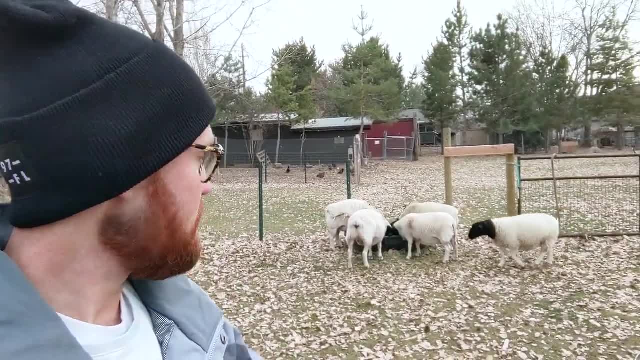 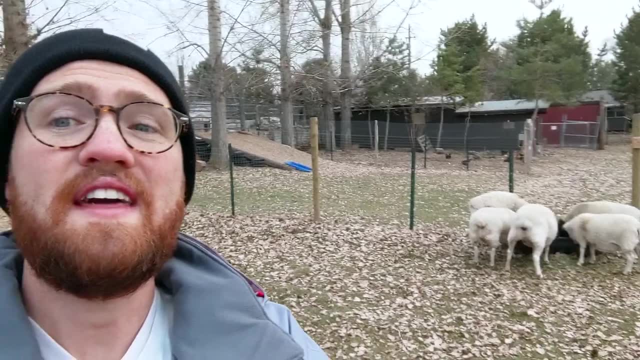 young, They're all in adolescence, right? This girl right there, for example, she's technically a lamb. She's about nine months old, Okay. So you see that and you look at her and you're like, Oh, she's not a baby. She looks to be the same size as the rest of them And the girl 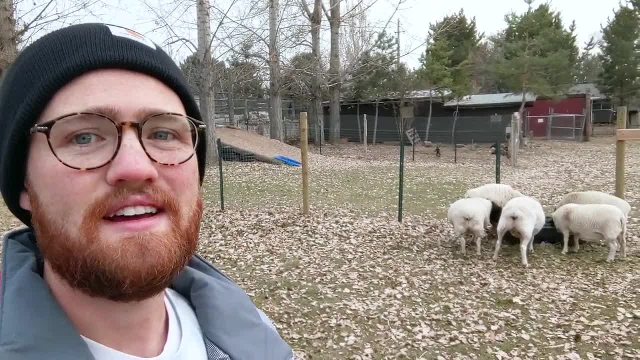 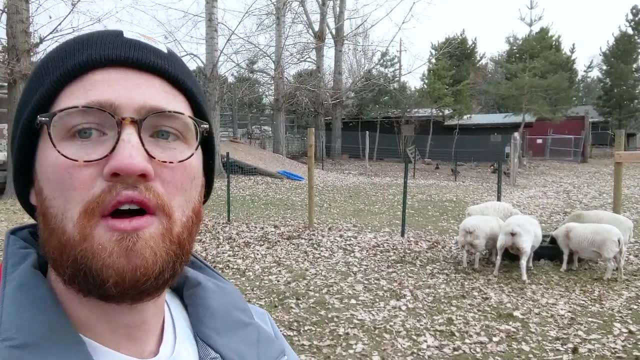 that she's next to. that's her mom. So you can see, uh, you can see the difference in size right there. It's not a tremendous difference. So when you hear about eating lamb or ordering lamb, you're not ordering. it's not. it's not the equivalent of veal, not the same thing, Okay So. 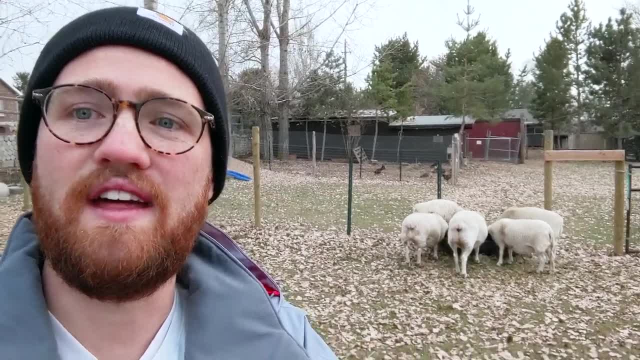 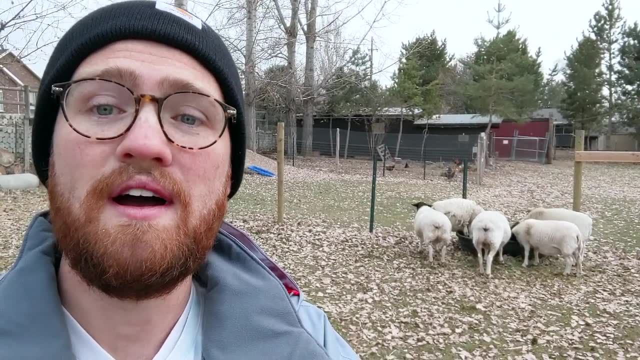 don't, uh, so don't don't be fooled into thinking that that it's that. I'm not saying: don't respect the life I absolutely do I've. I respect it more now after being part of the system, Um, but just. 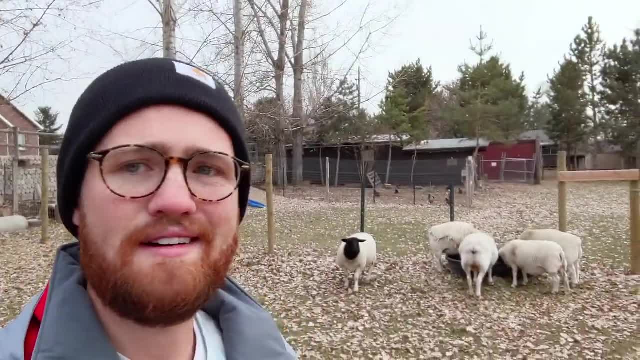 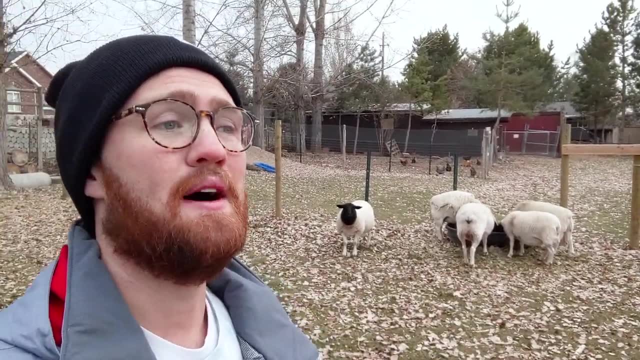 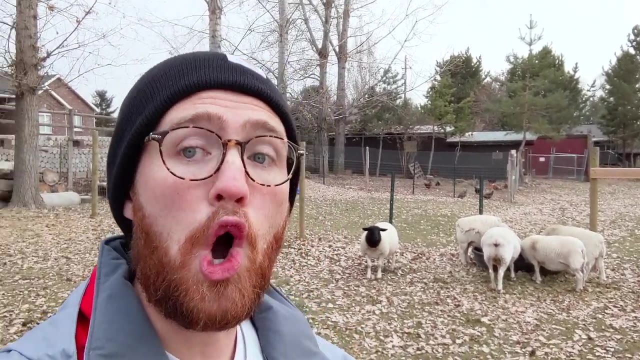 know that it's more adult than you think it is. Okay, That was a tangent, because that wasn't even in my script. What I wanted to say is that general rule of thumb with lamb- um, anything under anything that's processed under a year, and mutton is anything that's processed over 24 months, or 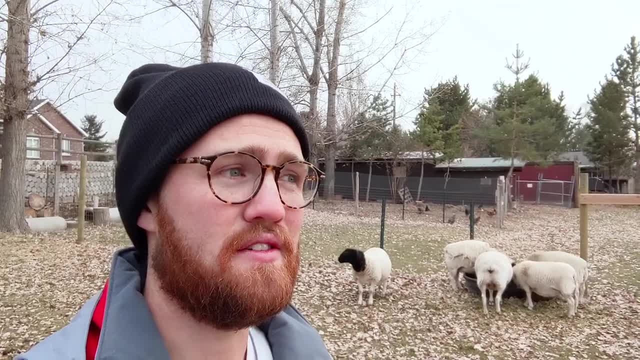 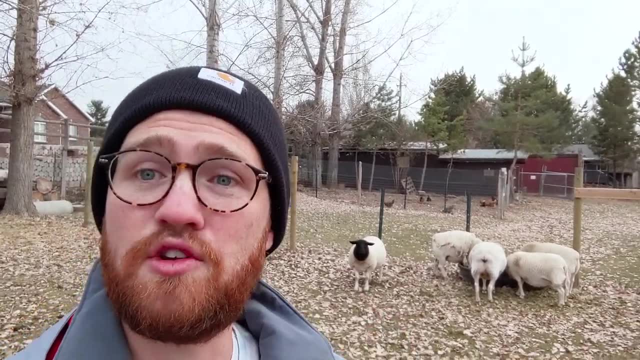 two years. So you look at that and you're like: all right, there's a year gap in that. So what happens if they're processed between a year and 24 months? And that's where the gray area comes in. So in the U S for the most part that's still. 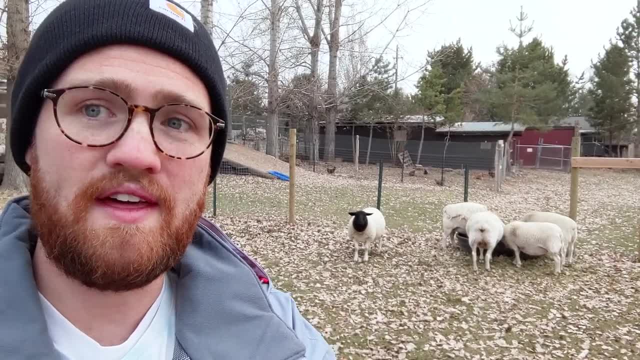 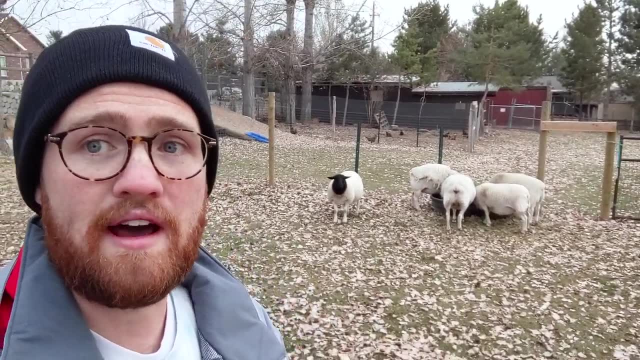 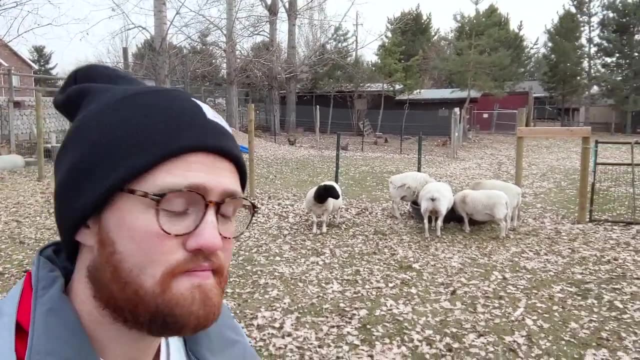 called lamb. So if you're at Costco or something like that and you see, you know rack of lamb, very likely that that lamb is over a year old. and I'm not knocking Costco. I think they do a better job than most uh, grocery stores and you know meat peddlers out there, But uh. 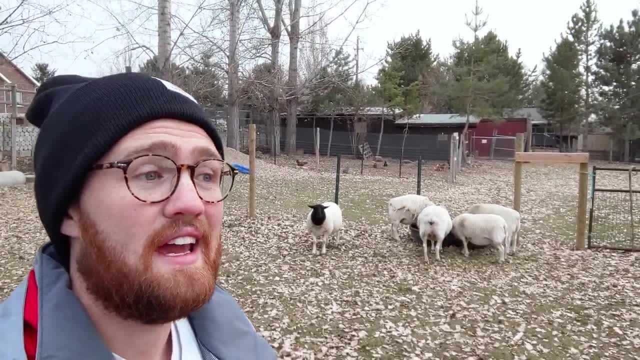 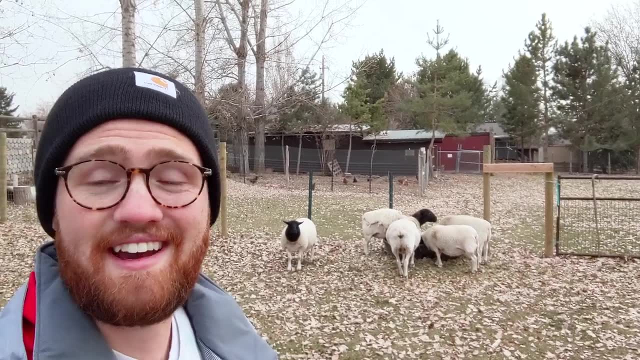 usually in the U S you're eating something that that's over a year old, And I think that's why so many people in the U S are like, oh, I don't really like lamb. It's like, well, you're not really eating the best quality. It's because people in the U S are too unaccustomed. 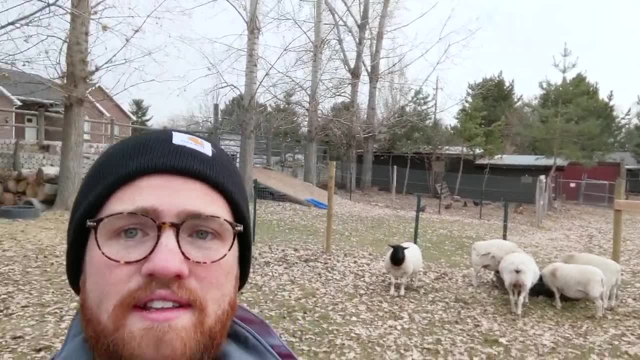 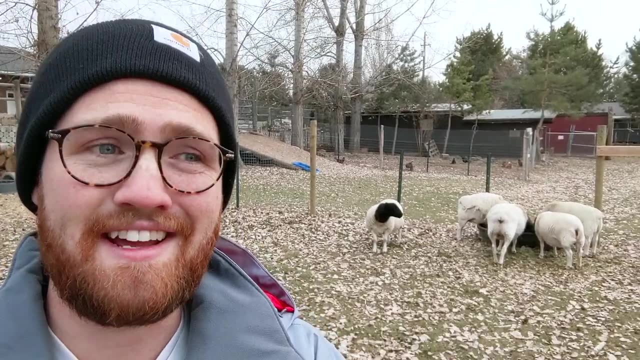 to it to know the difference. However, in Commonwealth nations, so that you know, UK, New Zealand, Australia, maybe Canada- I know Canada is a commonwealth, but I don't know if they do this. Um, but there's. 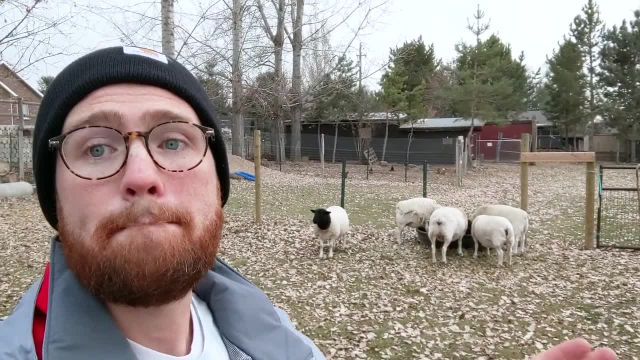 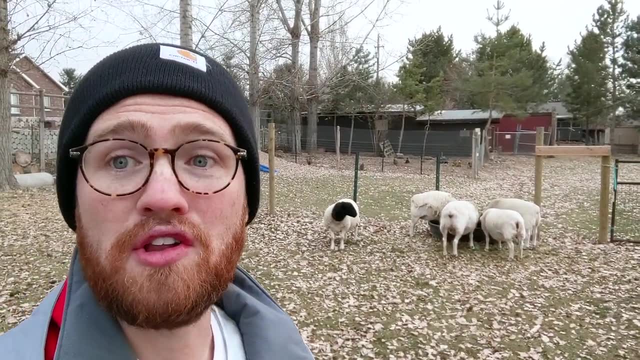 a third category. So there's lamb- anything under a year, uh, mutton- anything over two years, And then you have this middle ground, uh, which is called hogget. So fun fact if you've ever seen the movie babe, which I know you. 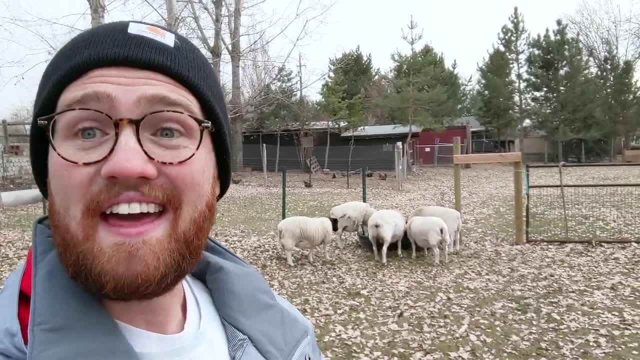 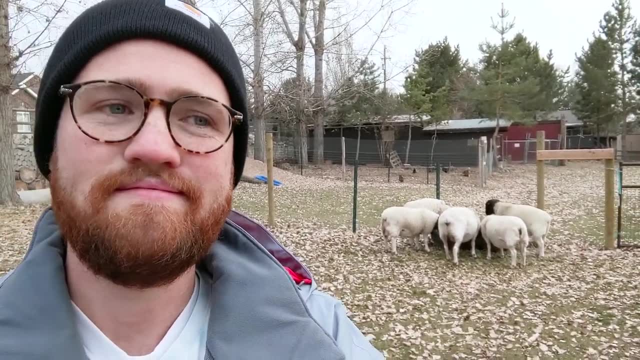 have cause babe's awesome. Um, that guy's name is farmer hogget And when I was a kid watching that, you know babe is the pig And so I thought hogget was a pun on. you know, oh, I get it like a pig. It's actually a sheep term, Um, so anything between uh. 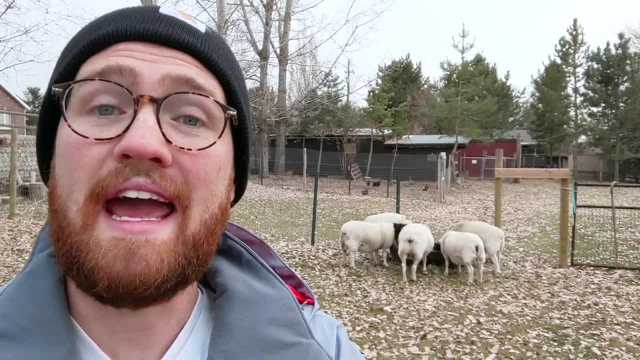 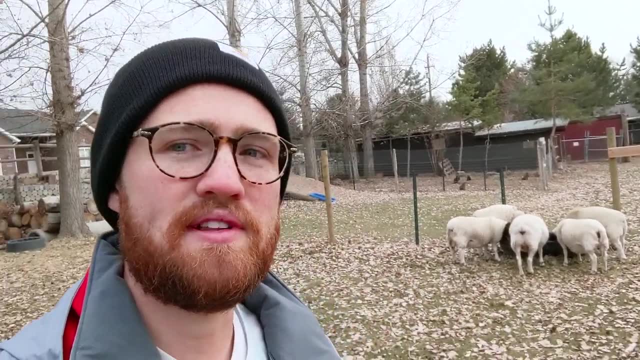 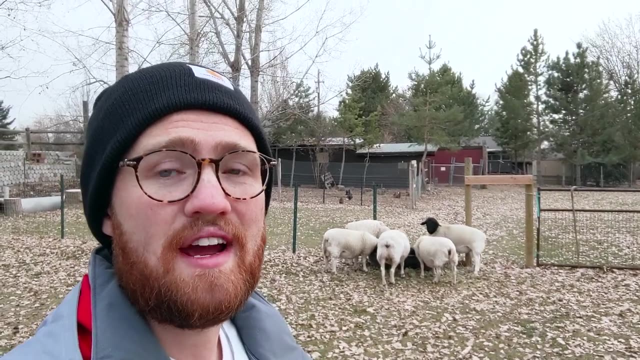 12 and 24 months at its processing age is hogget in the Commonwealth nations. I've also heard it called yearling Um, but that's mostly known by producers. Producers call it yearling, Not necessarily the consumer. Again, like I was saying, many people that try lamb in 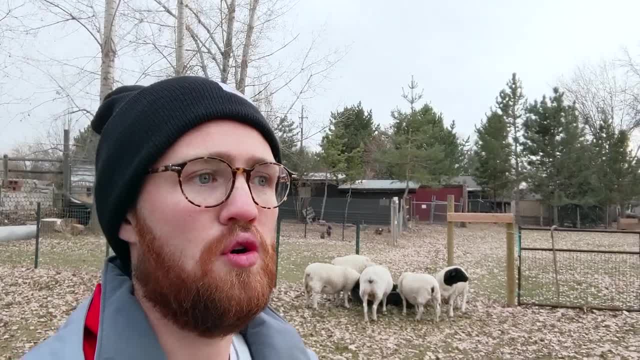 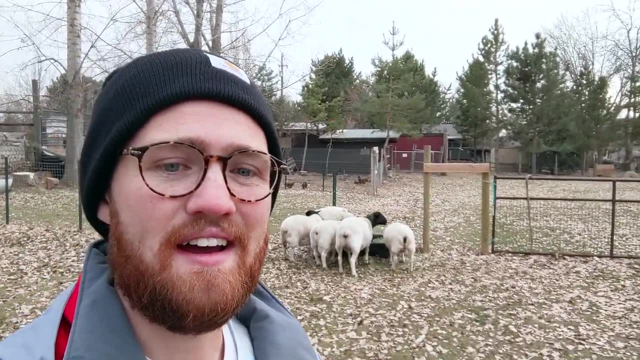 the U S especially, are trying lamb that is over a year old. So in my opinion that is not true lamb. So when you get that reputation like oh it's gamey, or I don't like the taste, uh, to be fair to you guys and to lamb producers like myself, you're not really trying true. 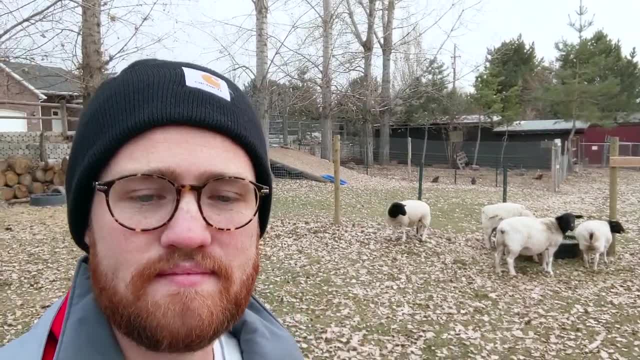 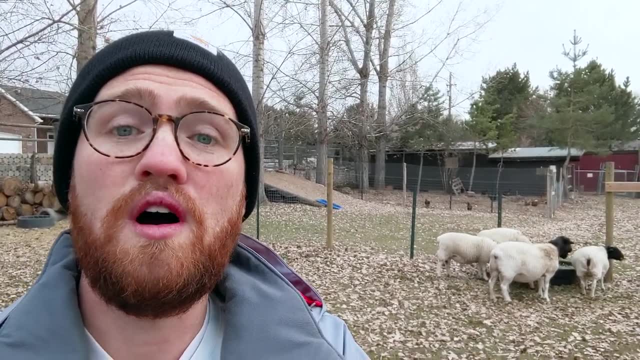 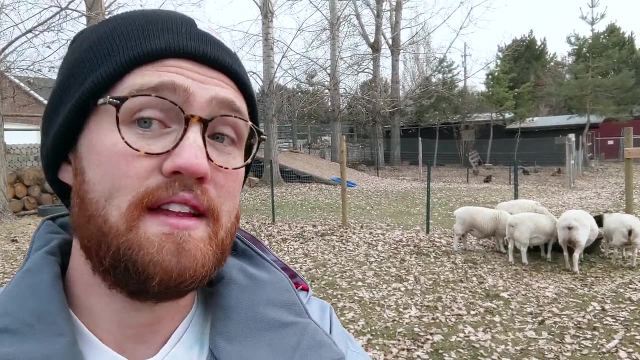 lamb- Well, that's glamorous right there. Nice, uh, poop or a pea shot while I'm talking about food, But you get the point. So, uh, look for local producers, Look for guys like me. Um, see if you can buy lamb- that is, that is true lamb- and see if that changes your mind. It. 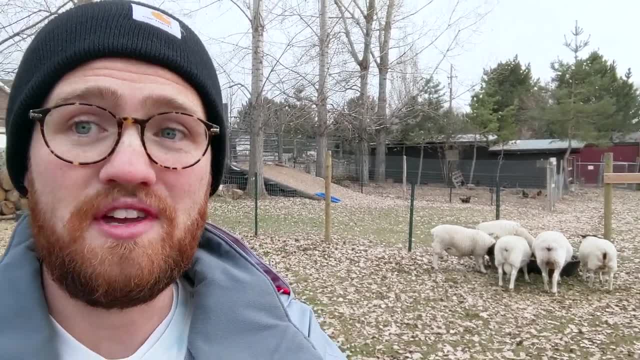 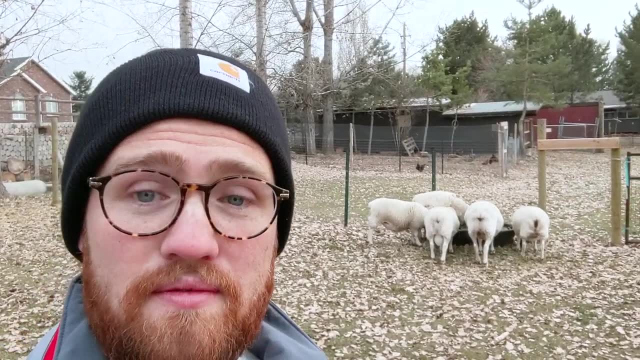 might not, but I guarantee you it's going to be better, Especially if it's Dorper, like these are. Hello, That's some good meat. I've converted many people to lamb with the Dorper. In fact, we're having- we're having lamb tonight, We're having lamb burgers, Hmm, So good. 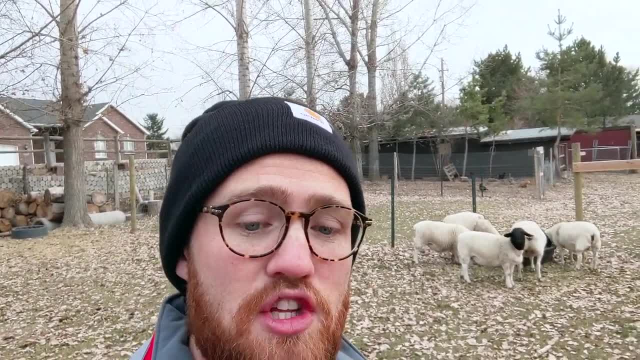 So, of course, local lamb is going to be the best lamb in the world. I mean, if you're a local producer, what are the best lamb that you're going to get? Well, I think I'm going to say the lamb that has the highest meat you can get, and that's because local 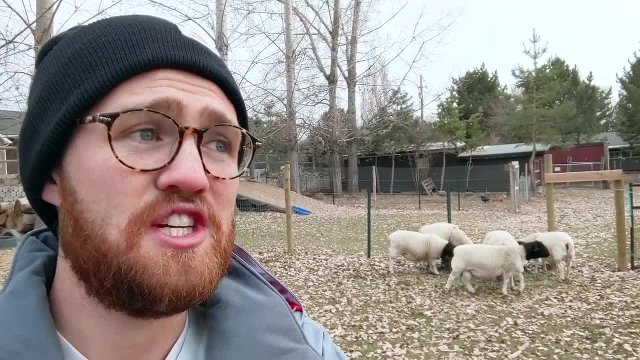 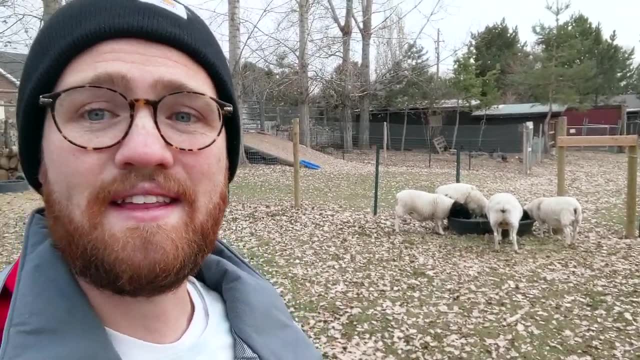 food is typically better cared for They're. they're out on pasture for the most part. Uh, sheep are supposed to be eating grass, and if they're hair sheep roughage also. So they're eating what nature intended them to eat and that's going to produce a better. 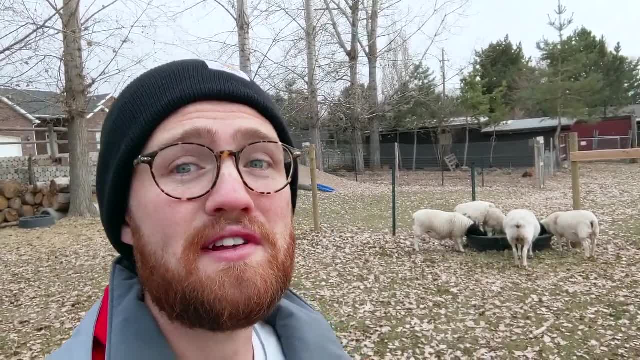 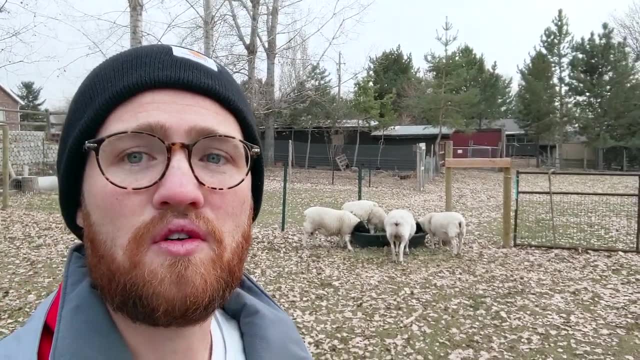 final product for you. But local food is also better, usually because they're getting processed at the appropriate time. Lamb producers are a good one, should take pride in food, But I, I don't know, I don't. I don't think that's a good thing. I think that's a good thing. 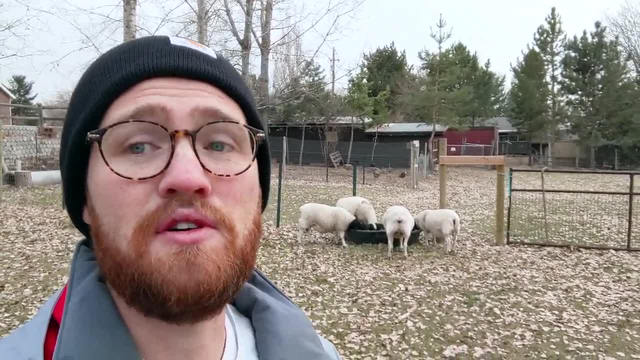 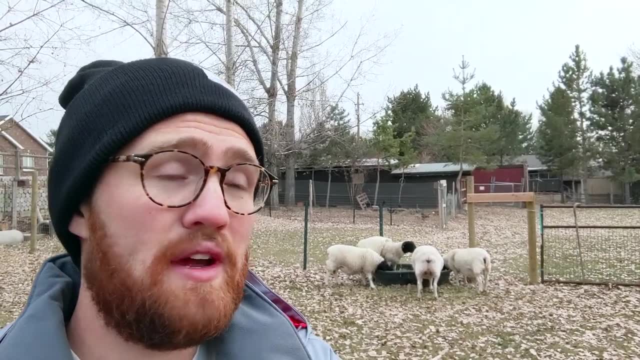 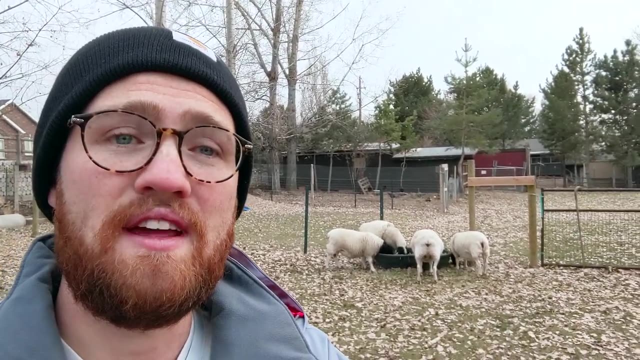 in the final product and what the taste is like, and that taste is influenced at processing time and the way that it is um that it's prepared beforehand. so, like me, they're eating grass and hay their whole life. i have done it both ways, i've done. i've done lambs with their last week. 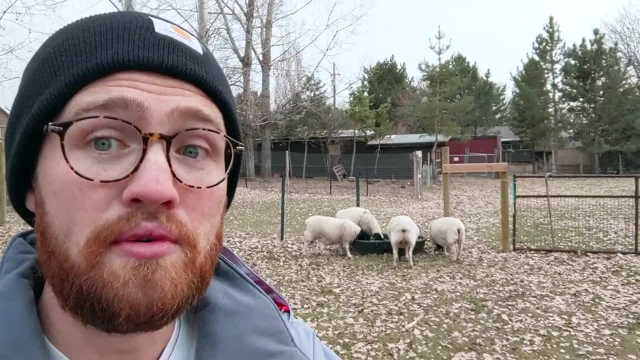 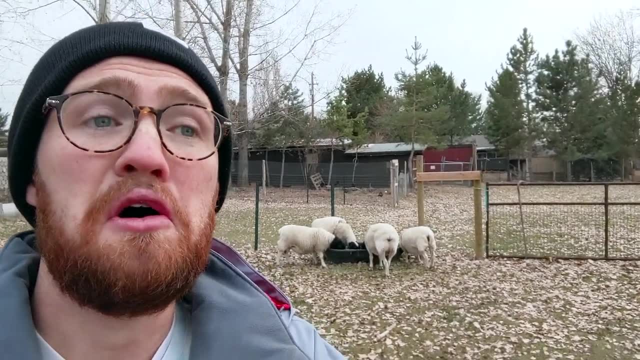 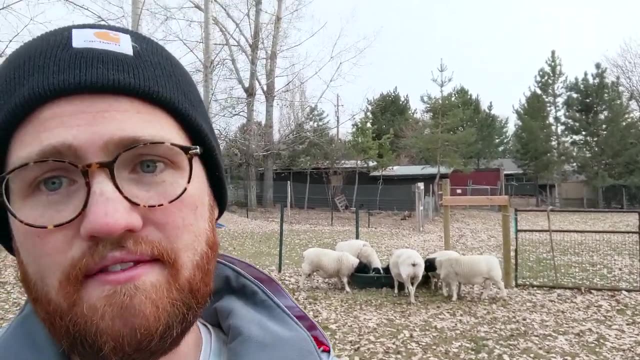 they get supplemented with maybe a cup a day of rolled oats, just to put on maybe like two or three more pounds um, and i've done it the other way also. so to me, like i'm, they're largely 100% grass fed, except maybe the last few days of their life here. so with local food you can also guarantee. 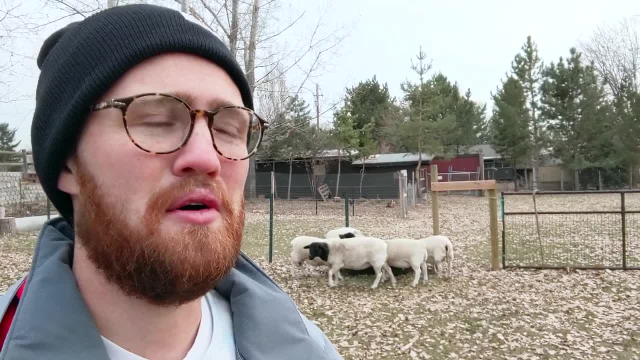 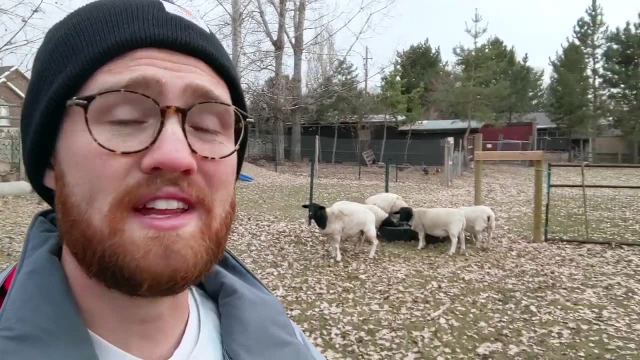 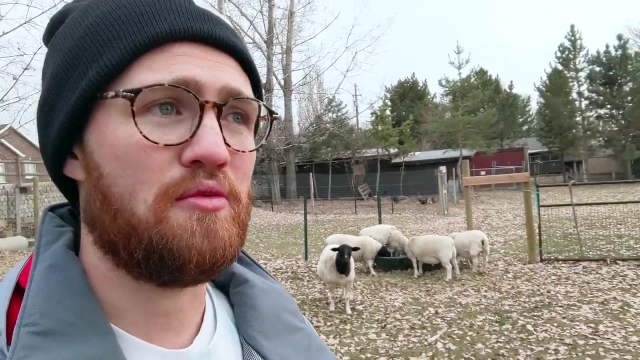 a healthier final product and it tastes better. so better taste, better health is better for your local economy. you're helping out someone that's doing something really important, because if you're using ruminants for what they're good for, which is on a farm like this, i feel like a broken record because you didn't come here to hear me rant about. 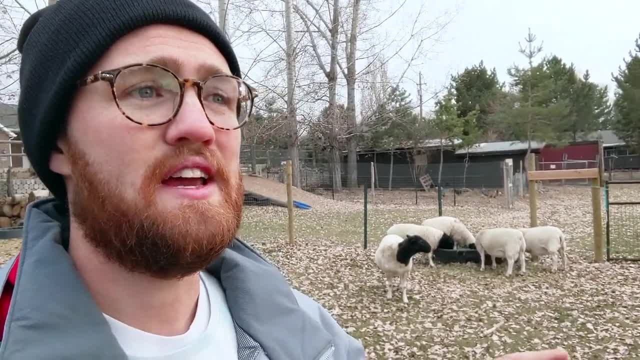 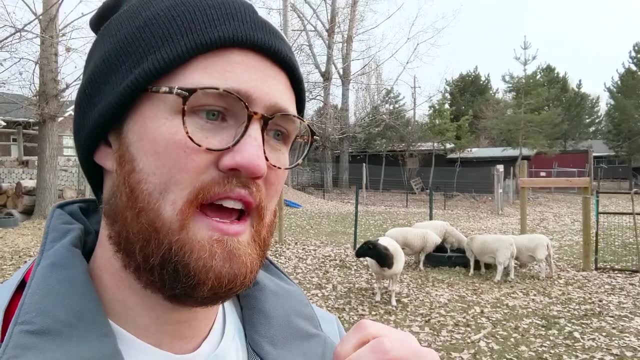 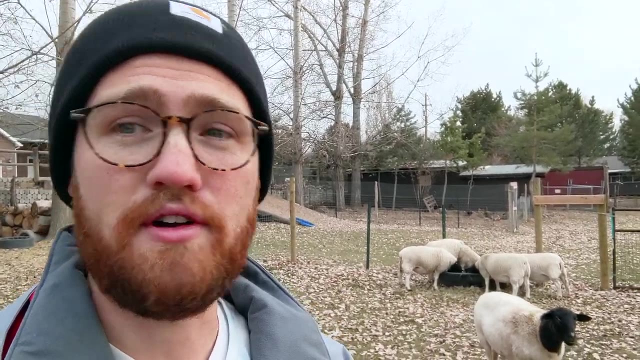 um the superpower of ruminants. but if you support local farmers doing this kind of thing, you're helping- uh, reverse climate change. you're sequestering carbon out of the air. you're doing all the right things. so please seek out local um local lamb producers. it'll change your mind.